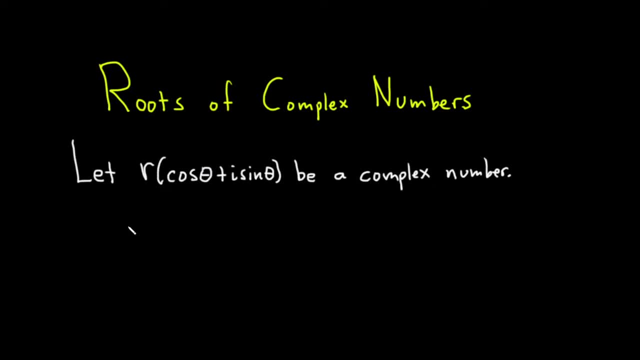 Theta is called the argument and r is called the modulus, And then we're going to let n be a positive integer. positive integer, Then our complex number, so our complex number, has exactly n distinct roots. So, for example, if n was 2, we would be talking about square roots, right? 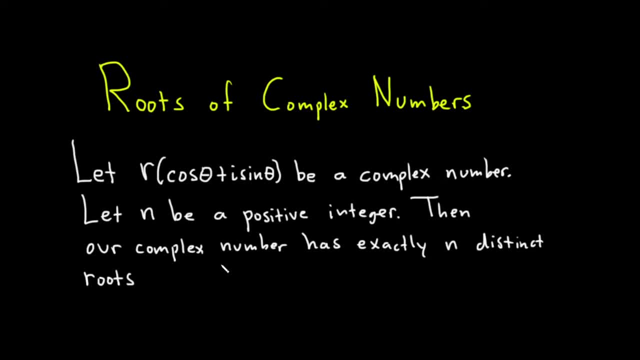 If n is 3, we're talking about cube roots. If n is 4, we're talking about fourth roots. n is 5, fifth roots, etc. So every number actually has two square roots. So then our complex number has exactly n distinct roots, given by 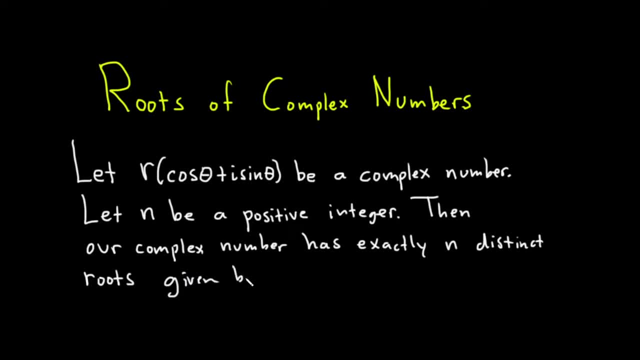 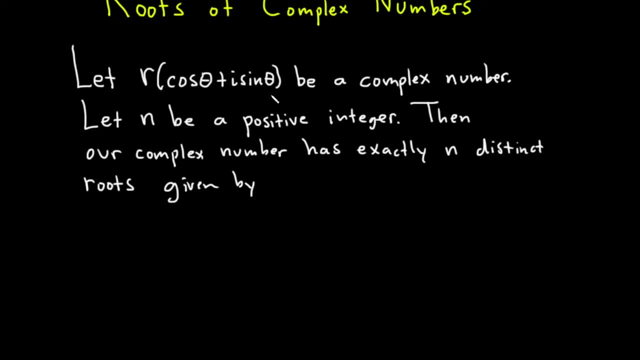 I'll give you the formula now given by, and I'm going to write the formula using: well, I guess I'll write it using this notation here first. So it's the nth root of the modulus times. let's use alpha, cosine of alpha, plus i sine alpha. 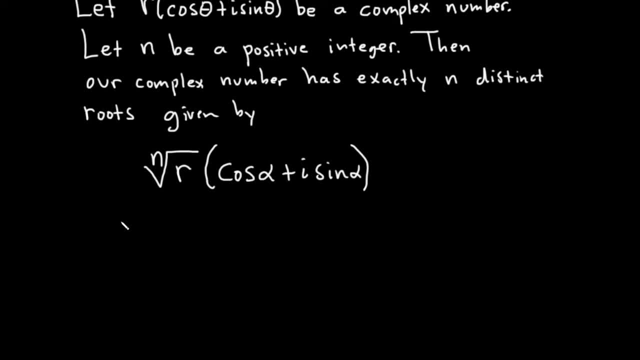 And what is alpha? So alpha here is going to be theta plus 2.5.. So it's going to be 2kpi divided by n, where a runs from 0 to n minus 1.. Okay, from 0 to n minus 1.. 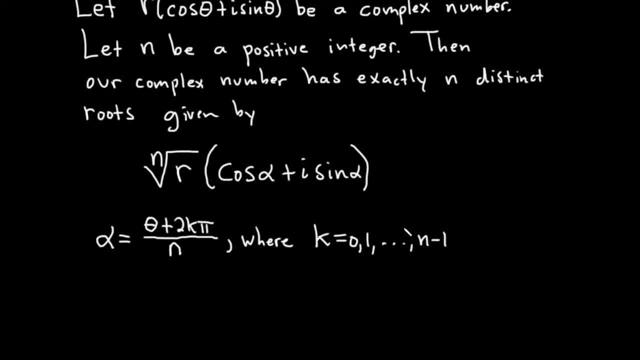 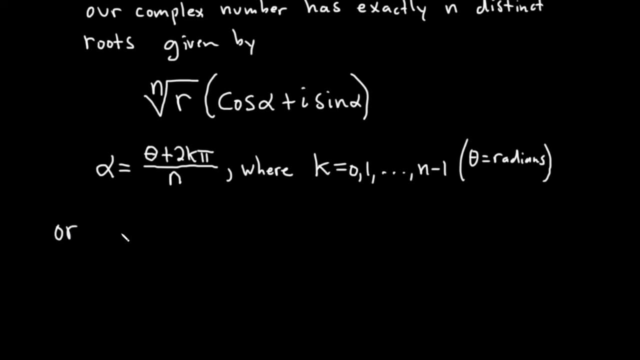 And here theta is in radians. So here theta is in radians. If theta is in degrees, the function is going to be: if theta is in degrees, the formula is very simple, very similar, rather, Or alpha equals theta plus. 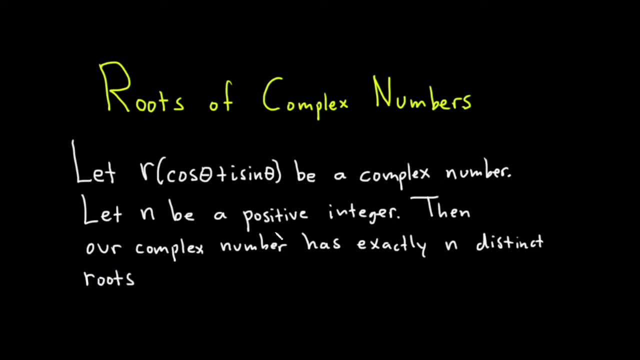 So, for example, if n was two, we'd be talking about square roots, right? If n is three, we're talking about cube roots. If it is f, we're talking about fifth roots. So every number actually has two square roots. 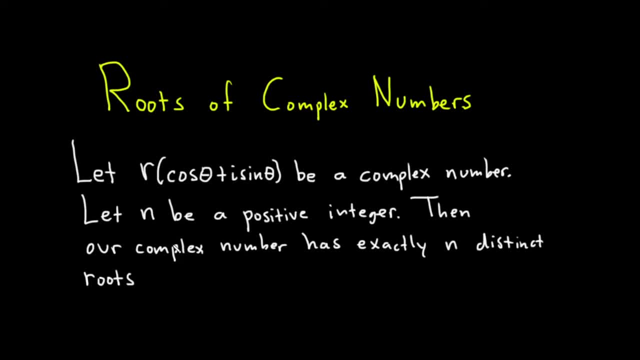 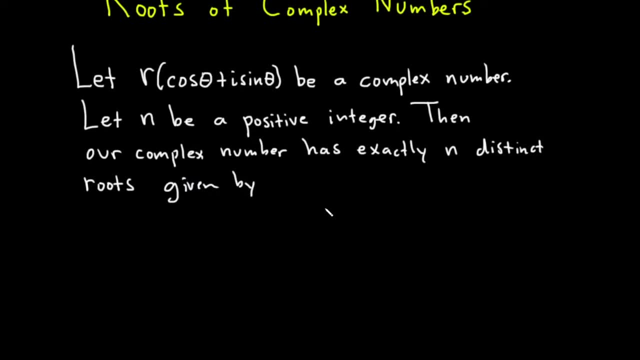 So then, our complex number has exactly n distinct roots, given by. I'll give you the formula now- is n. give it a formula now, given by, and i'm going to write the formula using: um. well, i guess i'll write it using this, this notation. 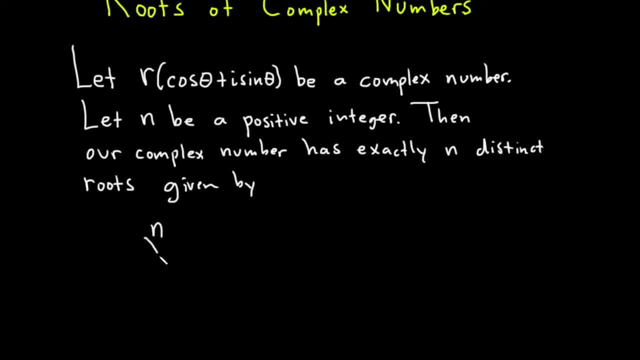 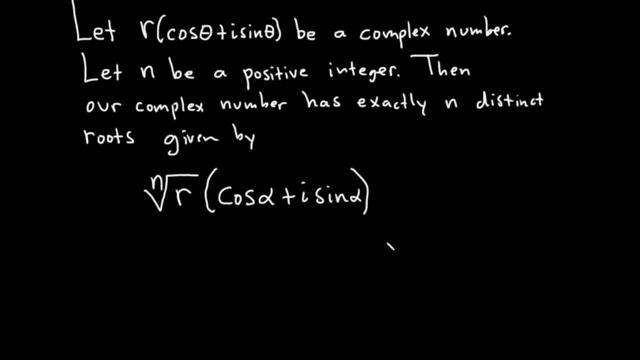 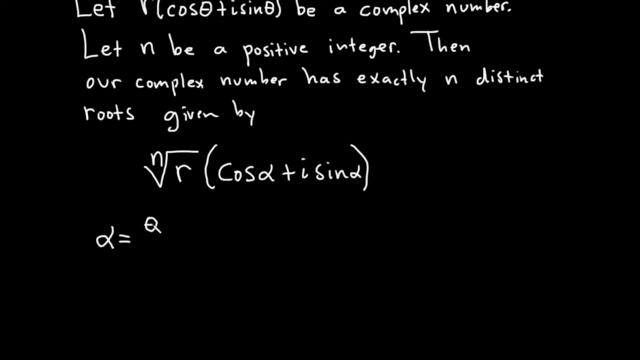 here first. so it's the nth root of the modulus times. uh, let's use alpha, cosine of alpha plus i sine alpha. and what is alpha? so alpha here is going to be theta plus 2k pi divided by n, where a runs from zero to n minus one. okay, from zero to n minus one, and here theta is in, uh, radians. 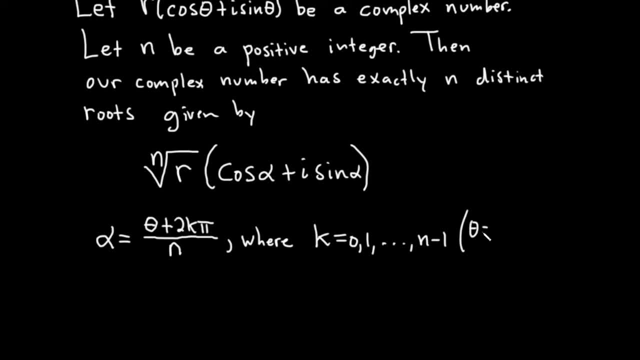 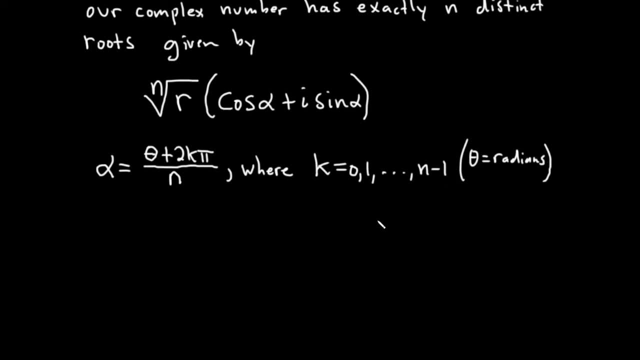 so here, uh, theta is in radians. if theta is in degrees, the formula is very simple, very similar. rather, uh or alpha equals theta plus. you simply replace the two pi with 360 degrees. so 360 degrees times k over n, and everything else is the same. so i'll i'll write it down here: 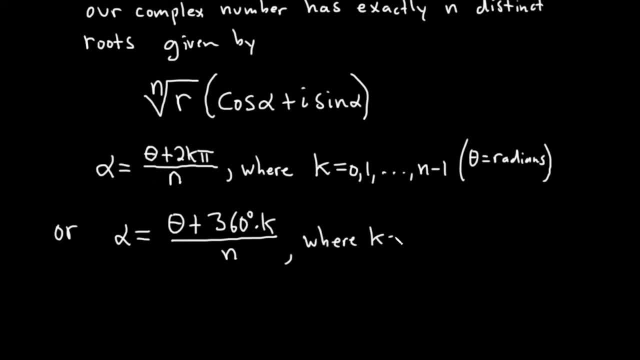 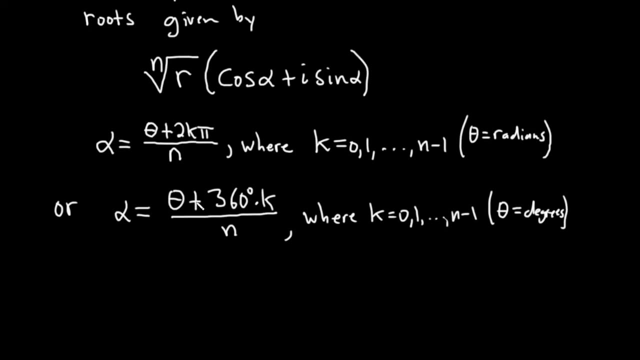 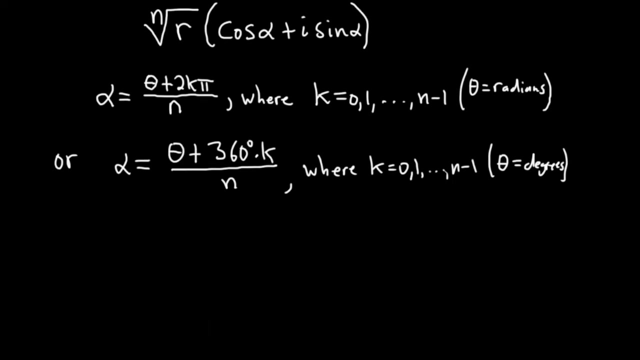 so let's just go ahead and do an example right away. um, so you see how to use this formula. i don't want to scroll down too much because i want to make sure you can see the formula on the screen. okay, so let's go ahead and do an example. so example. 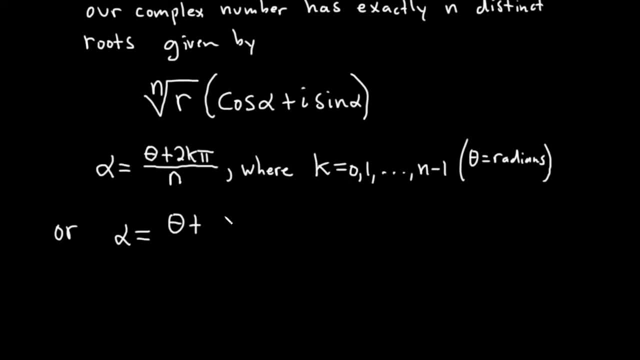 you simply replace the 2pi with 360 degrees, So 360 degrees times k over n, And everything else is the same. so I'll write it anyways, where k runs from 0 to n minus 1. And in this case theta would be in degrees. 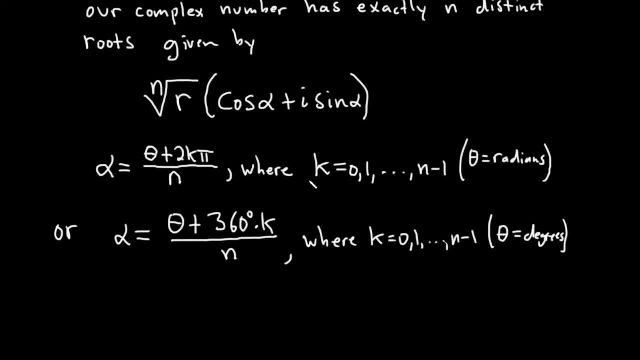 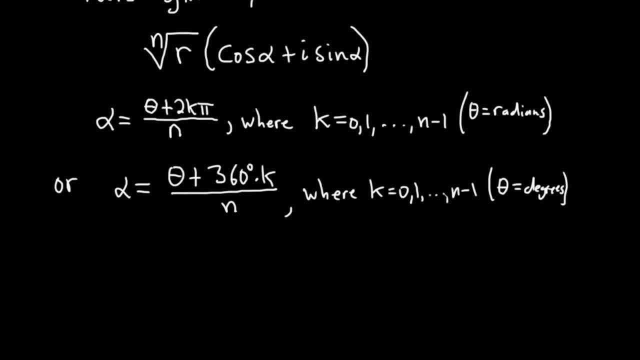 So let's just go ahead and do an example right away, so you see how to use this formula. I don't want to scroll down too much because I want to make sure you can see the formula on the screen. Okay, so let's go ahead and do an example. 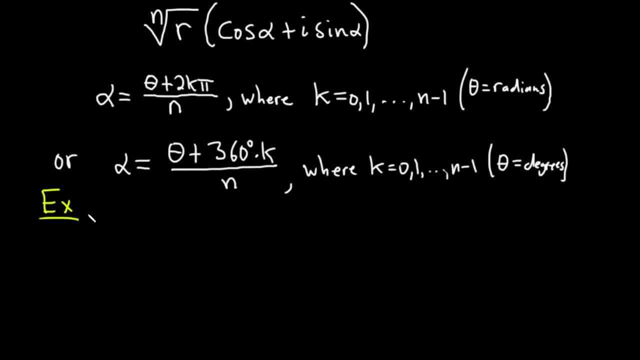 So example, And let's maybe just start off simple: We'll find the square roots of 4i. So find the two square roots. I'll just say the square roots. there's two of them, square roots of 4i. 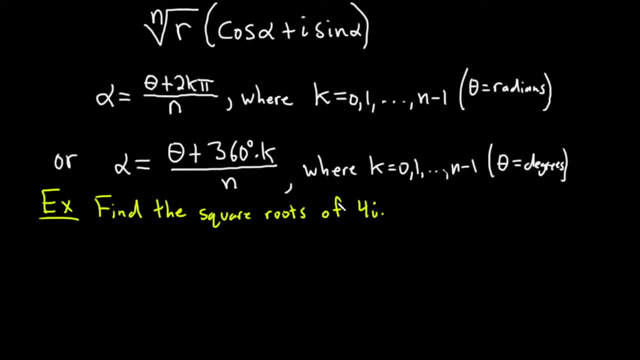 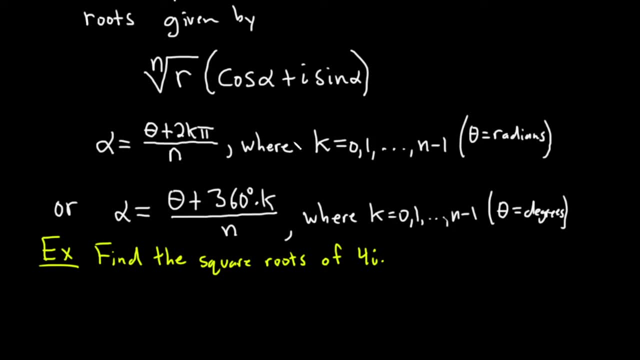 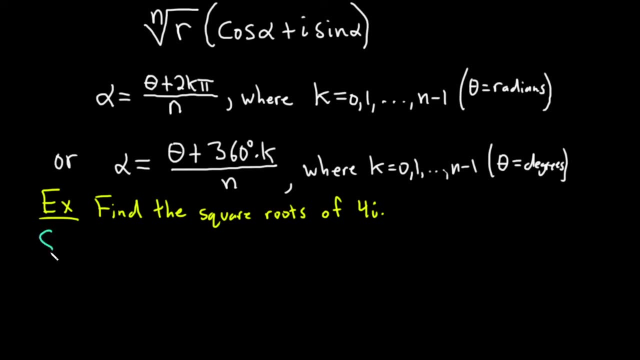 So you'll notice that in this formula up here the complex number was written in polar form. so a good first step would be to do that, would be to write 4i in polar form, which is also called trig form. So solution. 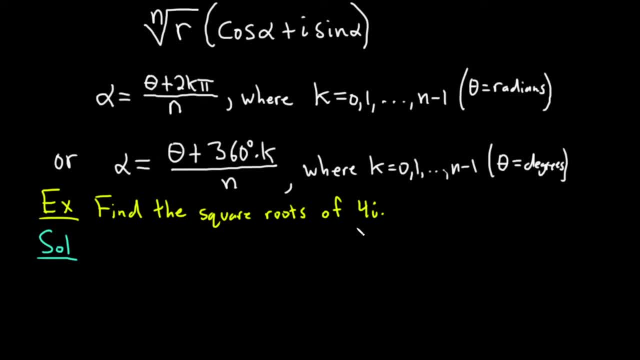 So there's a couple different ways to write this. in polar form, I think maybe the easiest way is to draw a picture. So 4i is here on the complex plane and r is the modulus, so r is this distance here, so r is 4.. 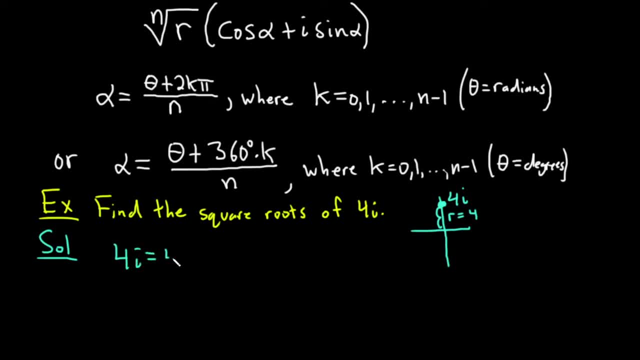 So 4i is equal to 4, that's your r parentheses, cosine theta. except what's theta here? right? Theta here is pi over 2, based off the picture plus i sine pi over 2.. Don't need an extra parentheses there. 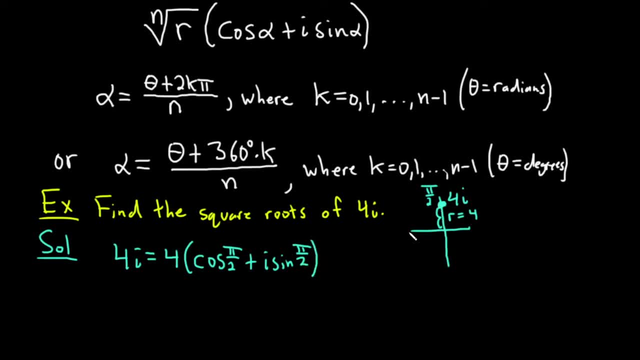 So whenever it's a quadrantal angle like this, for your theta it's very easy, like 4i, 2i, 3, you know, things that lie on either the x-axis or y-axis, any complex number that lies on an axis. 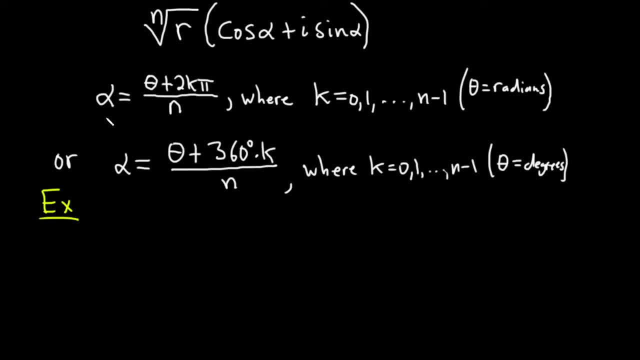 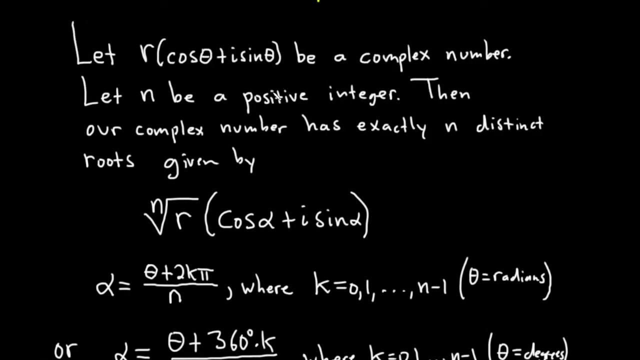 and let's maybe just start off simple. we'll find the square roots of 4i. so find the two square roots. i'll just say the square roots. there's two of them square roots of 4i. so you'll notice that, uh, in this formula up here, um, the complex number was written in polar. 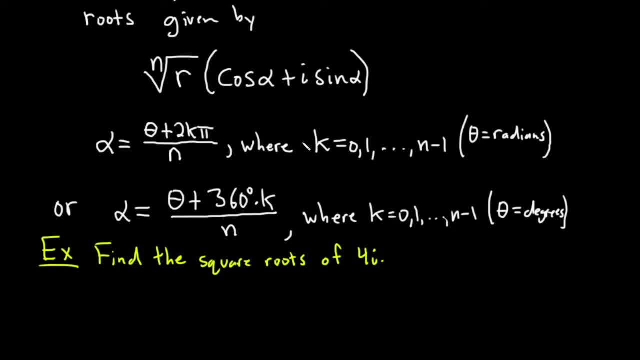 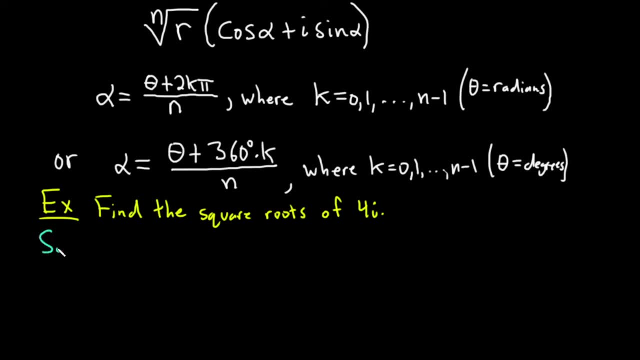 form. so a good first step would be to do that, would be to write 4i in polar form, which is also called trig form. so solution: so there's a couple different ways to write this in polar form. i think maybe the easiest way is to draw a picture. so 4i is here on the complex plane and r is the modulus. so r is this distance here. so 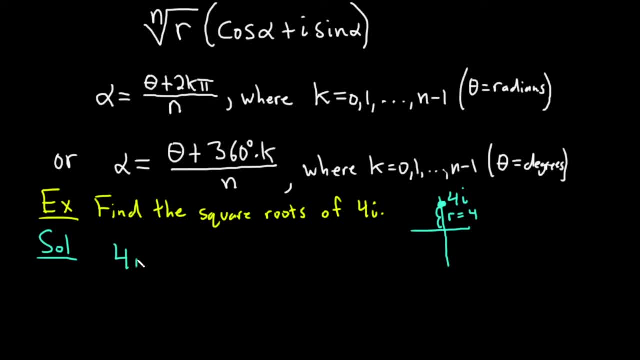 r is four, so four i is equal to four. that's your r. parentheses: cosine theta. except. what's theta here? right? theta here is pi over two, based off the picture plus i sine pi over two. don't need an extra parentheses there. so whenever it's a quadrantal angle like this, 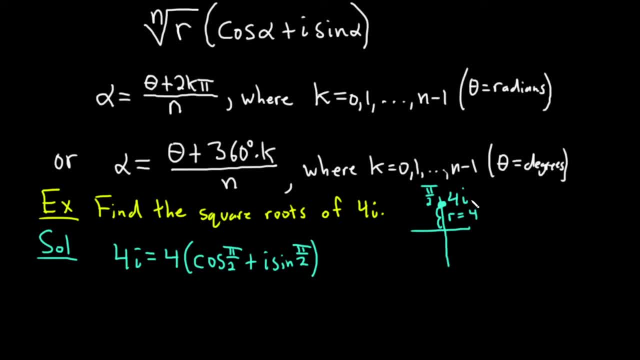 for your theta. it's very easy, like 4i, 2i, 3, um, you know, things that lie on either the x-axis or y-axis. any complex number that lies on an axis is very easy to write in polar form, because you can just draw a picture and you'll. 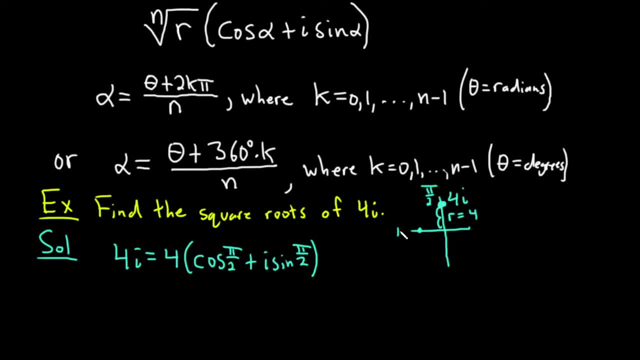 get the argument right away. for example, maybe it's over here. in this case, the argument is pi. maybe it's over here. in this case, the argument is three pi over two. maybe it's over here. in this case the argument is zero. so very easy when the complex number uh lies on one of these axes. 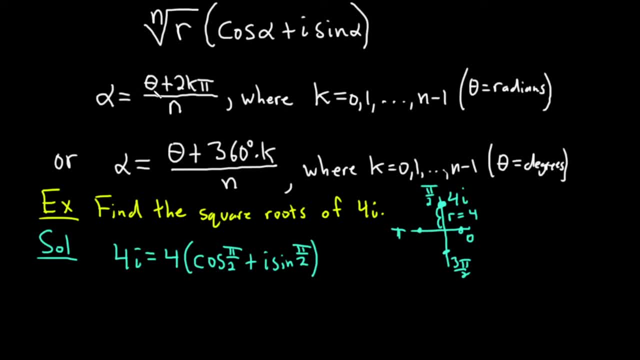 so that's the polar form. okay, that's the polar form. so now we just have to use the formula. so all we're doing here is using the formula. so here's our formula. so we need the nth root of R, so n here is 2, because we're looking for square roots, so the square 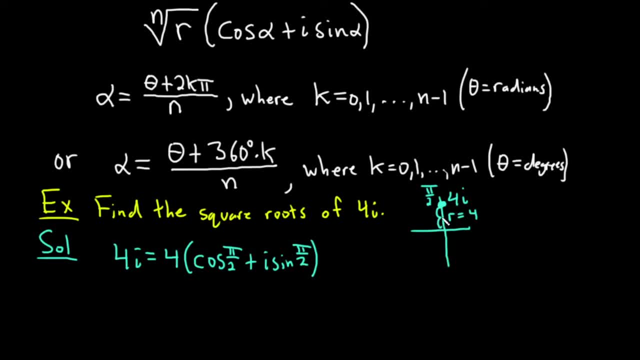 is very easy to write in polar form, Because you can just draw a picture and you'll get the argument right away. For example: maybe it's over here. In this case, the argument is pi. Maybe it's over here. In this case, the argument is 3pi over 2.. 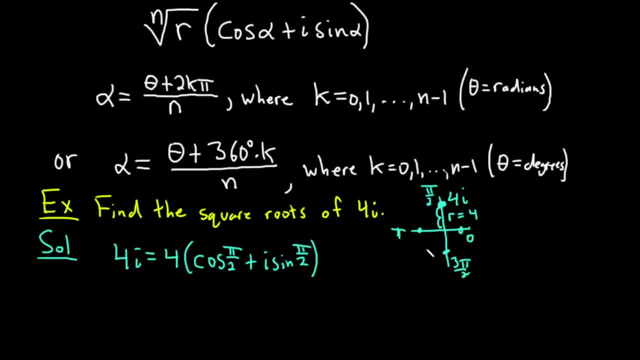 Maybe it's over here. In this case, the argument is 0. So very easy when the complex number lies on one of these axes. So that's the polar form. Okay, that's the polar form. So now we just have to use the formula. 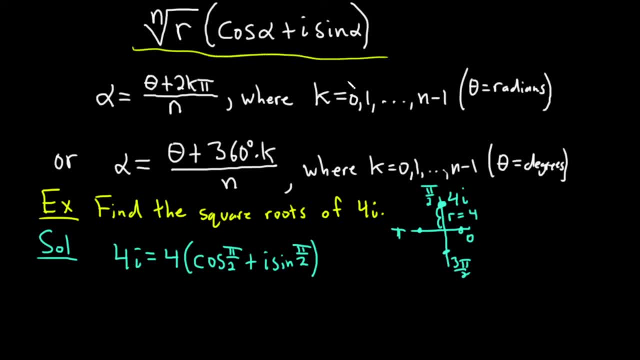 So all we're doing here is using the formula. So here's our formula. So we need the nth of r, So n here is 2, because we're looking for square roots, So the square root of r, r is 4,. 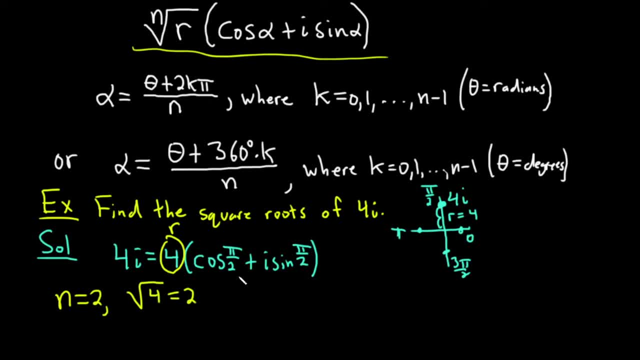 is 2.. Okay is 2.. And so now we just need to figure out alpha. So alpha is equal to theta plus 2kpi. So theta here is pi over 2.. That's our theta. It'll be pi over 2. 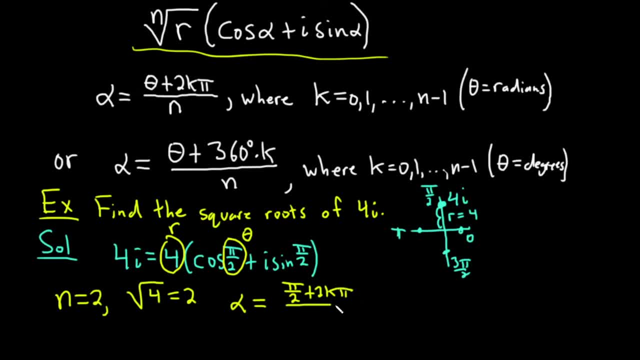 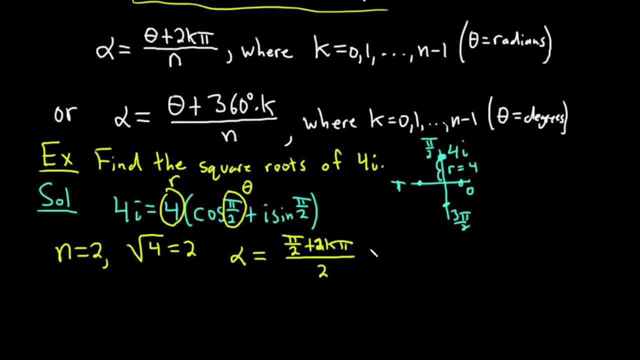 plus 2kpi Over n And again n, here is 2.. It's a 2 there. I hope you can see that 2kpi. So let's just find the different values now. So let's see. 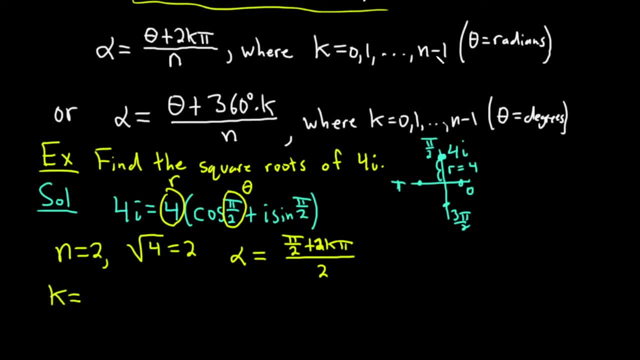 When k is Well, k runs from 0 to n minus 1.. So k is either 0 or 1, right, Because n is 2. So k is 0 and 1.. So when k is 0,, 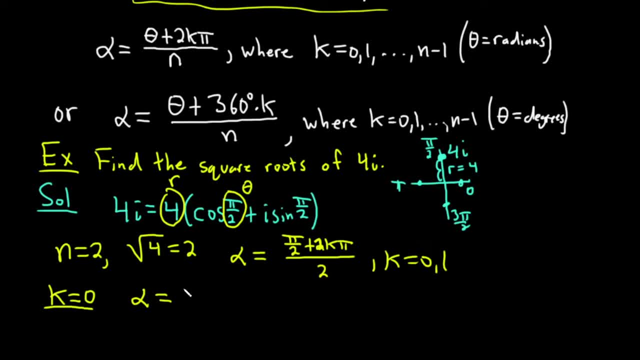 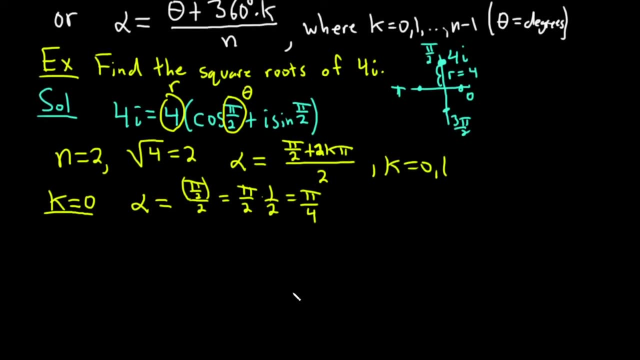 alpha equals. Well, that's going to go away, So we'll just get pi over 2.. over 2, which is really pi over 2 times 1 half, which is really pi over 4.. And when k is equal to 1,. 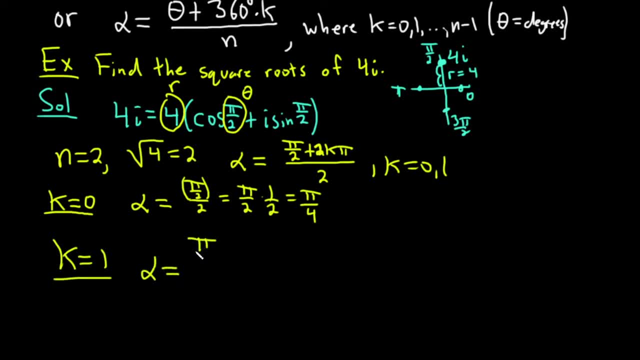 we get alpha equals would be pi over 2, plus k is 1, so you just get 2pi and all of that is divided by 2.. So this is pi over 2. And we're adding 2pi to it. 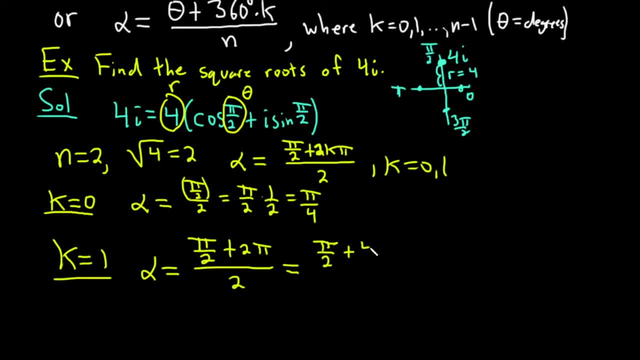 So think of 2pi as a number over 2.. One way to do that would be 4pi over 2. And that's over 2.. Going a little fast here with the adding of the fractions Pi over 2 plus 4pi over 2 is 5pi over 2.. 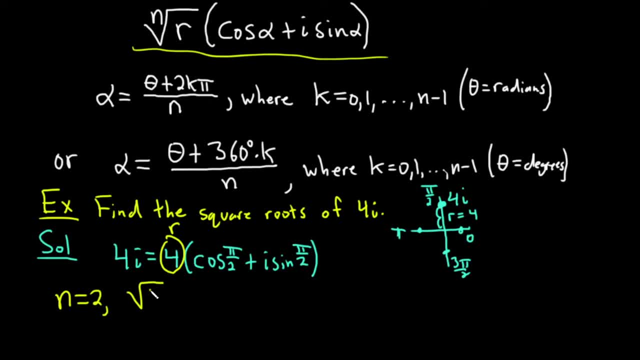 root of R, R is 4 is 2, okay is 2, and so now we just need to figure out alpha. so alpha is equal to theta plus 2k pie. so theta here is pi over 2. that's our theta. we pi over 2 plus 2k pi over n, and again n here is 2. it's a 2 there. hope you can. 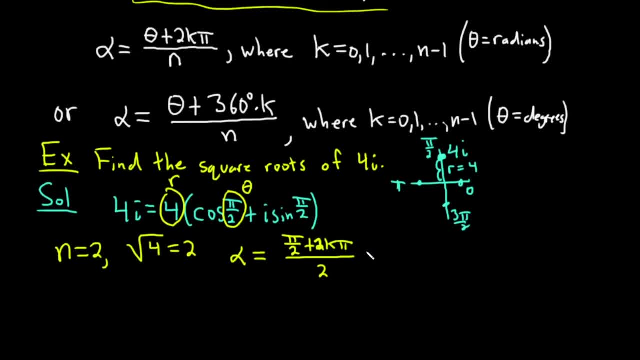 see that 2k, pi. so let's just find the different values now. so let's see when K is well, K runs from 0 to n minus minus 1.. So k is either 0 or 1, right, Because n is 2. So k is 0 and 1.. So when k is 0, alpha. 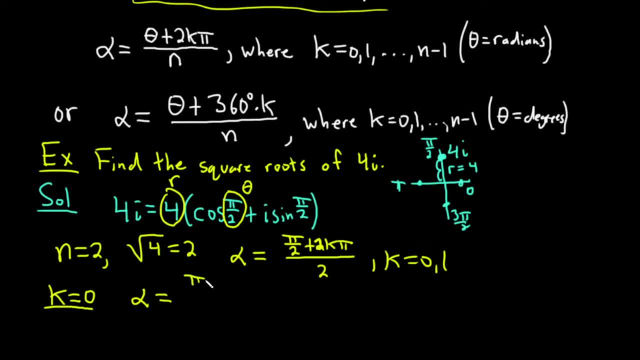 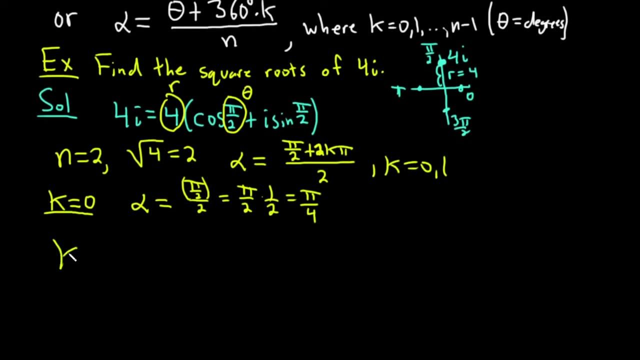 equals. well, that's going to go away. So we'll just get pi over 2 over 2, which is really pi over 2 times 1 half, which is really pi over 4.. And when k is equal to 1, we get. 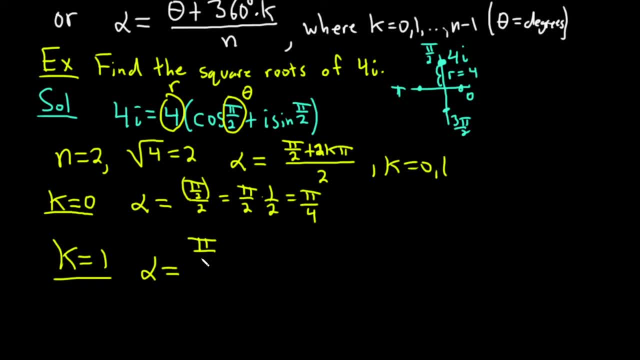 alpha equals would be pi over 2, plus k is 1.. So you just get 2 pi and all of that is divided by 2.. So this is pi over 2, and we're adding 2 pi to it. So think of 2 pi. 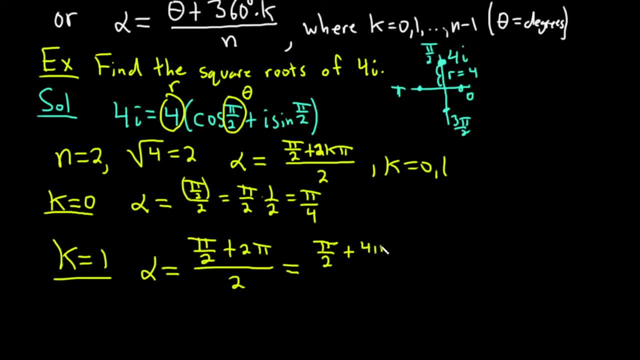 as a number over 2.. One way to do that would be 4 pi over 2, and that's over 2.. Going a little faster with the adding of the fractions Pi over 2 plus 4 pi over 2 is 5 pi over 2.. 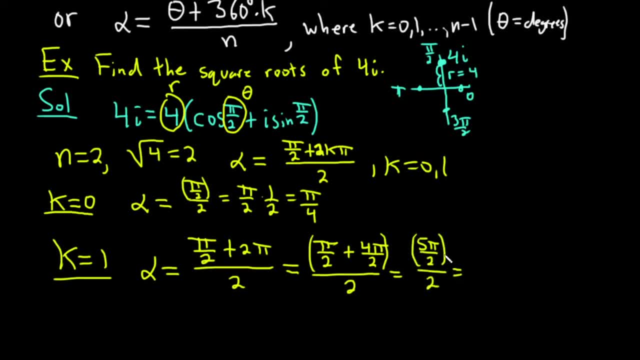 And all of that's over 2.. 5 pi over 2 divided by 2 is the same thing as 5 pi over 2 times 1 half, That's 5 pi over 4.. So those are our two angles: pi over 4 and 5 pi over 4.. And 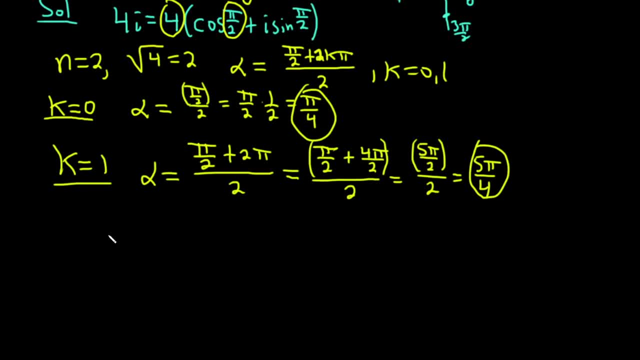 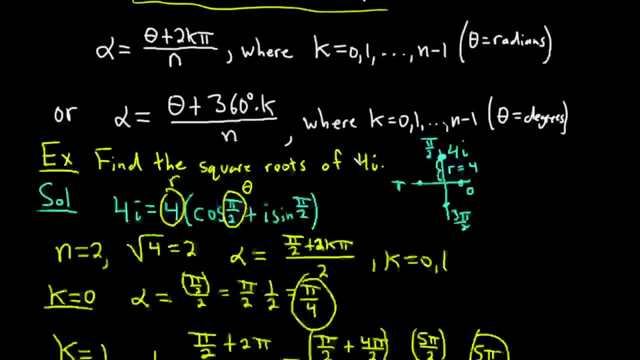 again the formula. I'll write it down for you, so you have it- is the nth root of r cosine alpha plus i sine alpha. That's the formula for the roots where alpha is given by this formula, The formula here which we just used, right? So we use the formula. So now all we do is: 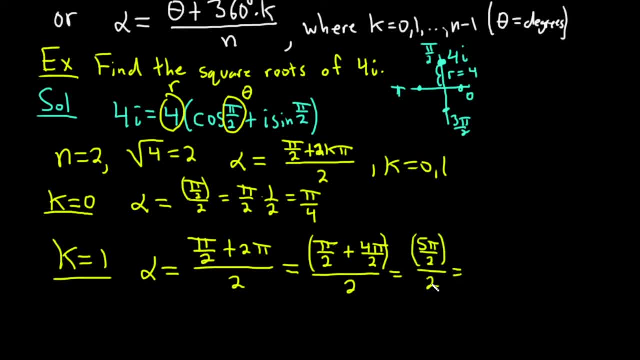 And all of that's over 2.. 5pi over 2 divided by 2 is the same thing as 5pi over 2 times 1 half, That's 5pi over 4.. So those are our two angles. 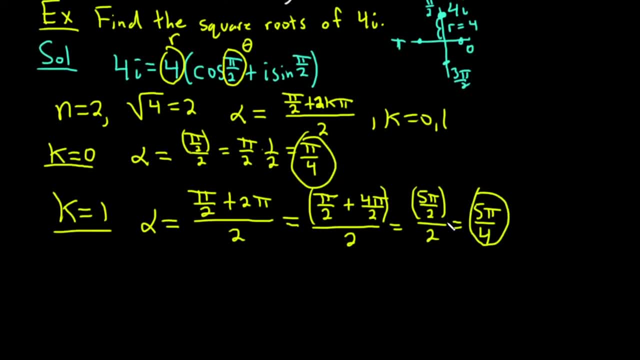 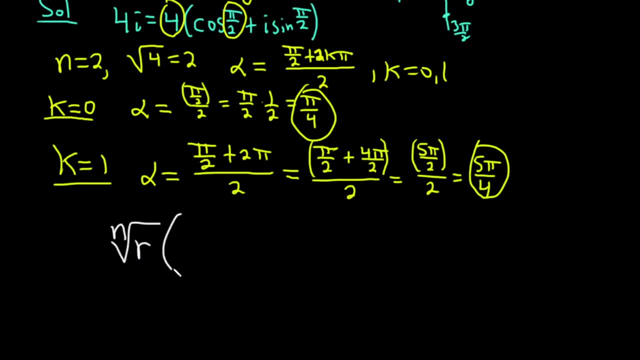 Pi over 4 and 5pi over 4.. And again the formula- I'll write it down for you, so you have it- is the nth root of r cosine alpha plus i sine alpha. That's the formula for the roots where alpha is given by this formula here. 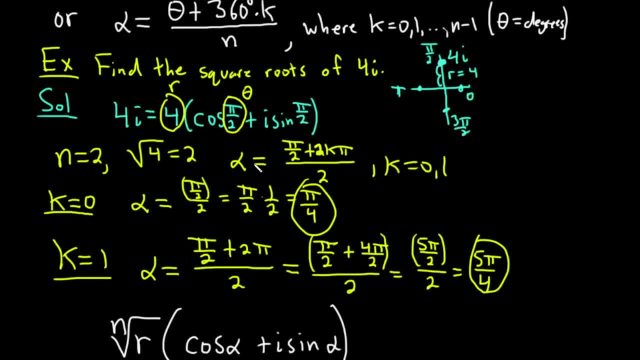 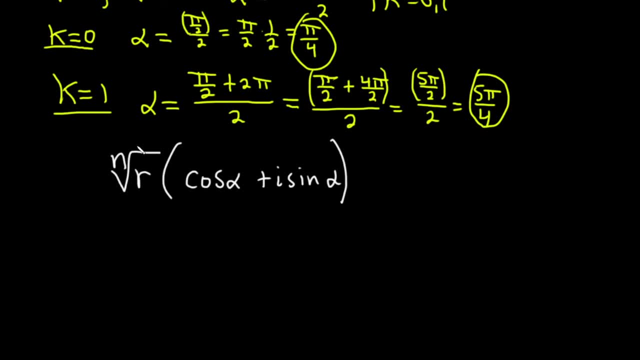 which we just used. right. So we use the formula. So now all we do is plug in the different values of alpha. So one of the square roots would be: Well, what was this here? This quantity here we said was 2.. 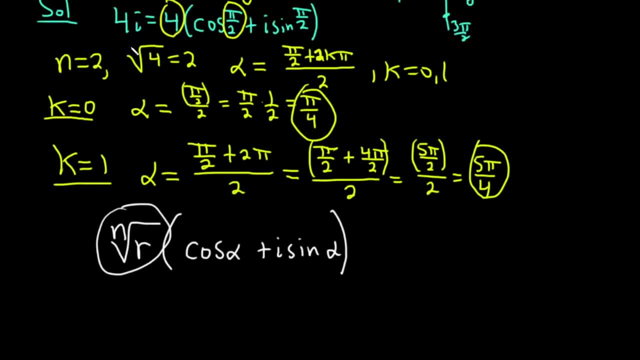 We did that here. There is an invisible 2 here. I'll write your r as 4.. So this is 2. Cosine of pi over 4 plus i sine of pi over 4.. So that would be one of the roots. 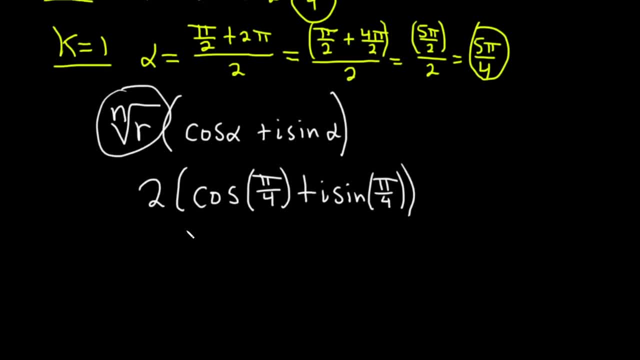 You could work this out. So this would be 2 squared of 2 over 2 plus i squared of 2 over 2.. Distribute the 2, and you simply get squared of 2 plus i squared of 2.. The 2s cancel. 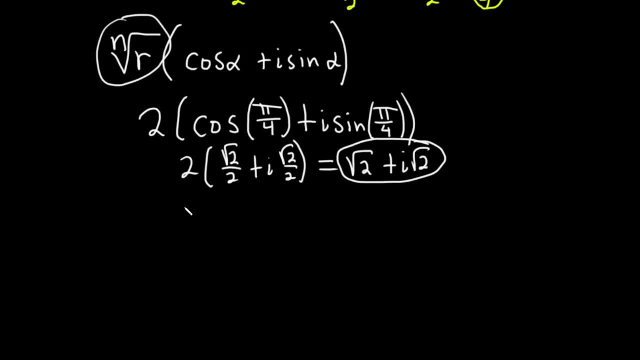 So that's one of the roots. The other root we would get by plugging in 5pi over 4.. So 2 cosines. You see these problems take a while and this is actually one. that's pretty simple. Plus i sine 5pi over 4.. 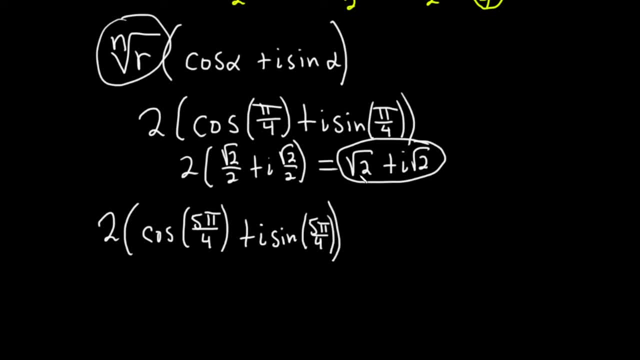 It's a pretty lengthy process. It's not hard, It just takes time. 5pi over 4, where is that? It's down over here, right, Because we can think of pi as 4pi over 4.. So if you go a distance of pi over 4. 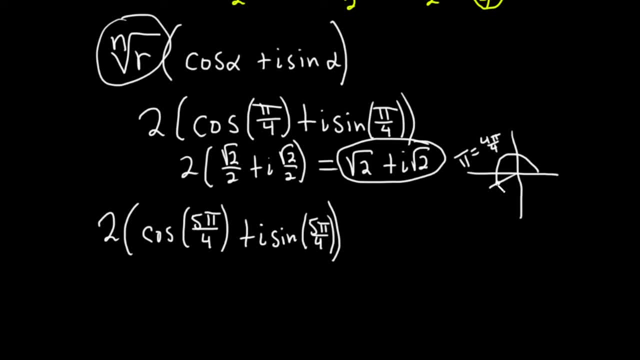 more than that. you're going to be down here in quadrant 3.. And here both cosine and sine are negative, because cosine is the x coordinate on the unit circle and x is negative here Sine is the y coordinate on the unit circle. 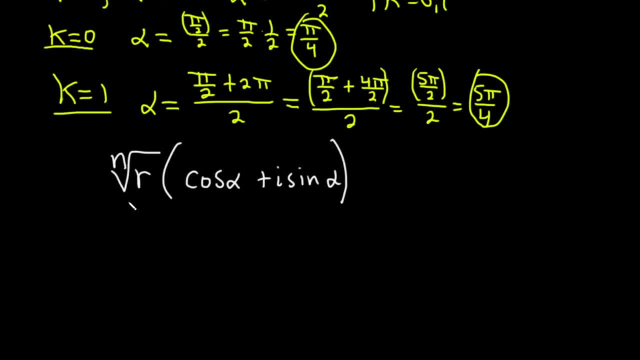 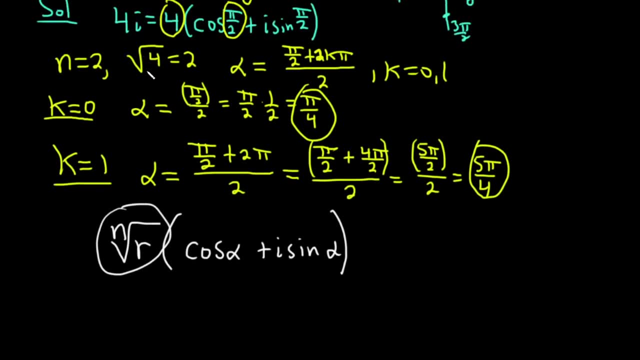 plug in the different values of alpha. So one of the square roots would be: well, what was this here? This quantity here we said was 2.. We did that here. There is an invisible 2 here. I'm going to write your r as 4.. So this is 2 cosine of pi over 4 plus i sine. 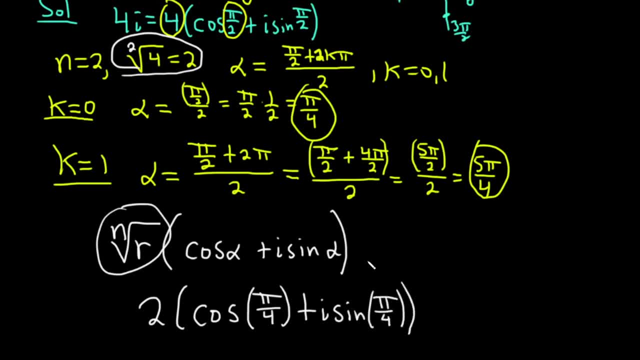 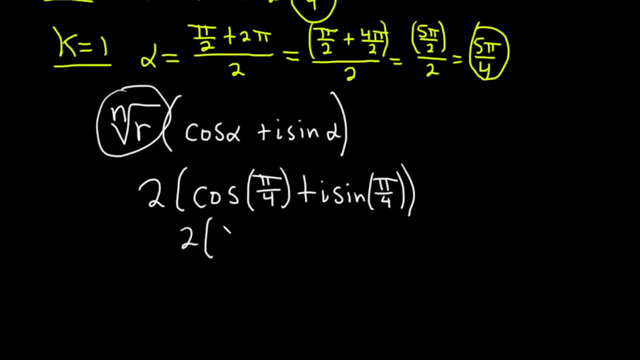 of pi over 4.. So that would be one of the roots. You could work this out. So this would be 2 square root of 2 over 2, plus i square root of 2 over 2.. Distribute the 2 and you. 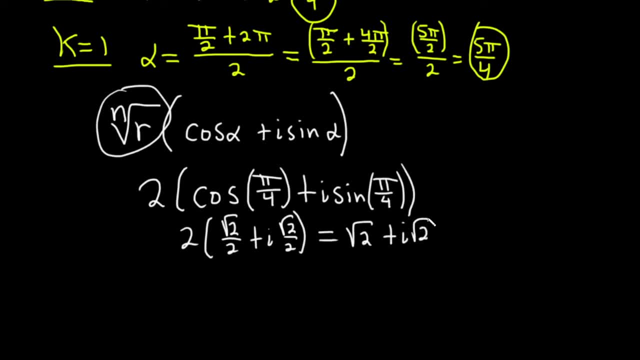 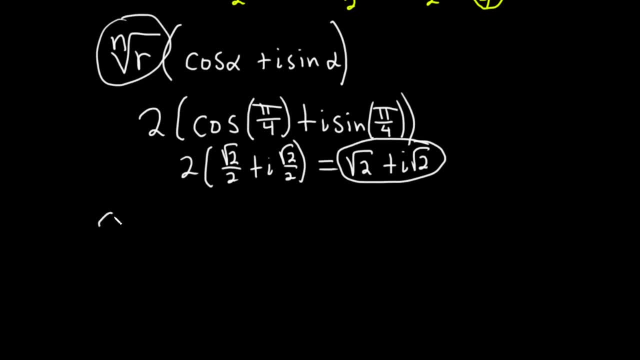 simply get square root of 2 plus i square root of 2.. The 2s cancel. So that's one of the roots. The other root we would get by plugging in 5 pi over 4.. So 2 cosine of pi. 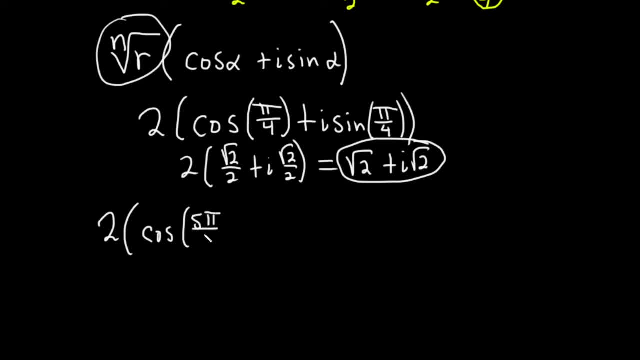 over 4.. You see, these problems take a while. This is actually one that's pretty simple. Plus, i sine 5 pi over 4.. It's a pretty lengthy process. It's not hard, It just takes time. 5 pi over 4, where is that? It's down over here, right, Because we can think of pi as 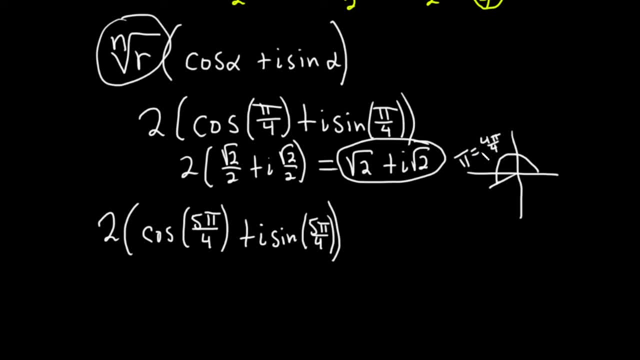 4 pi over 4.. So if you go a distance of pi over 4, more than that, you're going to be down here in quadrant 3.. And here b, Both cosine and sine are negative because cosine is the x-coordinate on the unit circle. 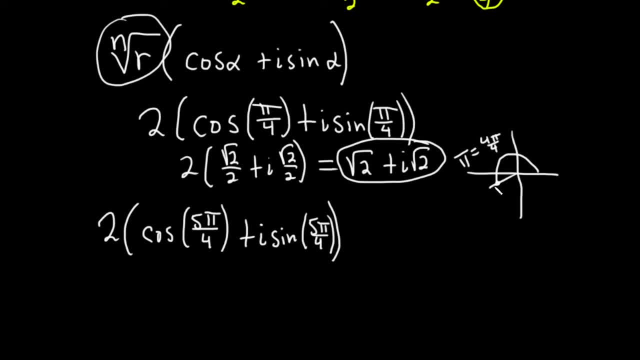 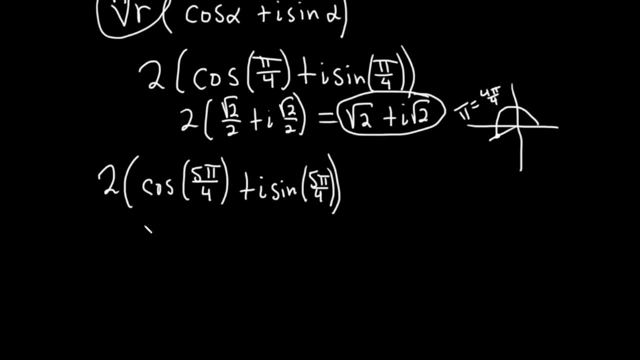 and x is negative here, Sine is the y-coordinate on the unit circle and y is negative there. So those are both going to be negative root 2 over 2.. So this is going to be 2 negative root 2 over 2, plus i negative root 2 over 2.. And then you distribute the 2 here And 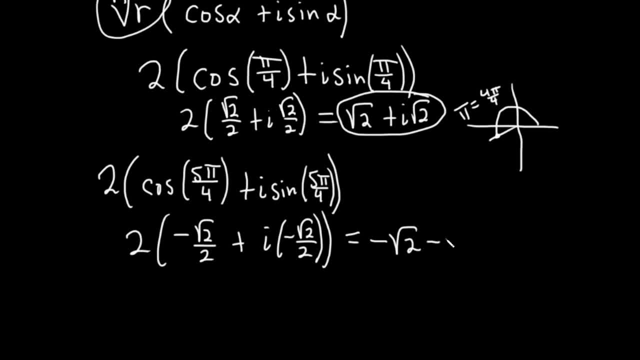 the 2s will cancel. You'll get negative square root of 2.. Minus i square root of 2.. So these would be the square roots. Both of these are the square roots of the pure imaginary number 4i. That's what these are. So we found the